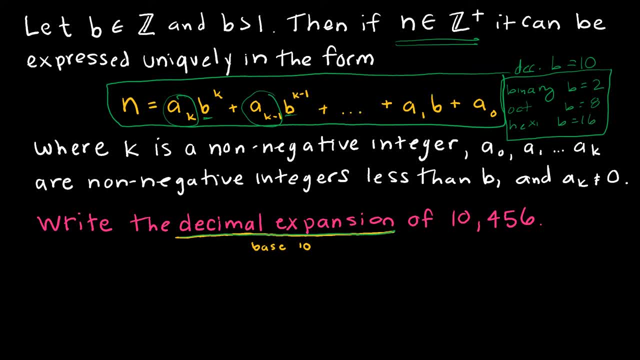 but in the expansion we're going to write a decimal expansion just for practice. So if I'm doing some examples that follow this, it will say: write something as a decimal expansion. Typically we're not going to write something base ten using the format that I'm going to show you. 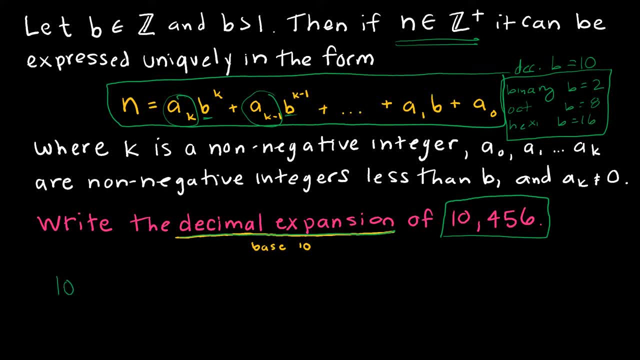 right now. This one's just for practice. So if I wanted to write 10,456 as a decimal expansion, I would say one is in the 10,000ths place. Well, this is a base ten number, right? So this is the ones place. that's ten to the zero. This is the tens place. this is the 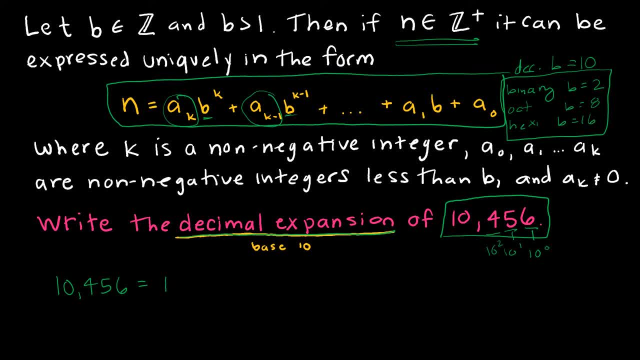 that's 10 to the first. This is the hundreds place, that's 10 squared. This is the thousands place, that's 10 to the third, And this is the 10 thousands place, or 10 to the fourth. So this is 1 times 10 to the fourth plus 0 times 10 to the third. 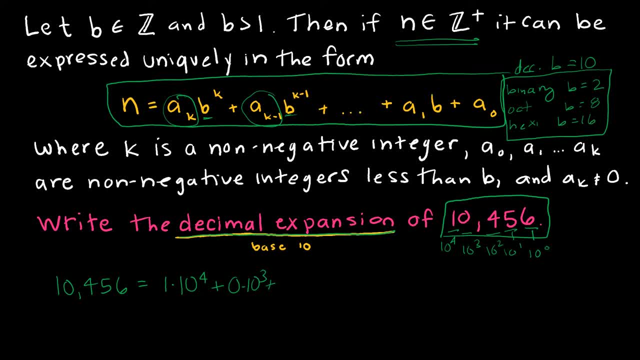 plus 4 times 10, squared plus 5 times 10 to the first, plus 6 times 10 to the zero. So if they really wanted me to write it as an expansion, this is what it would look like. But again, in the next examples that we do, it will say: write it as an expansion, And I'm just 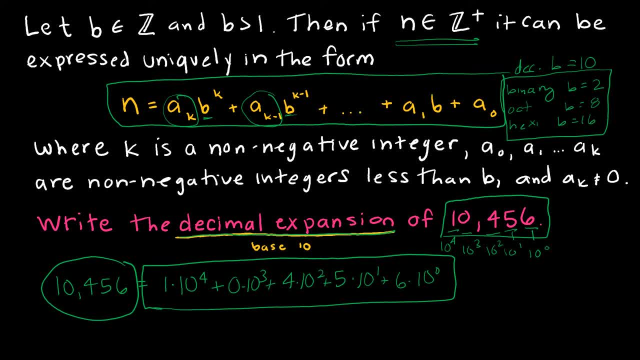 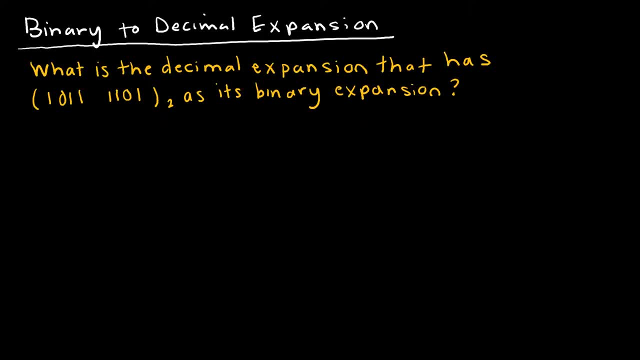 going to write a solution that looks like this, And that's pretty standard for decimal expansion, because that is the format of values that we are used to. So let's look first at binary to decimal expansion, And you may or may not be familiar with the binary system. Binary is made up: 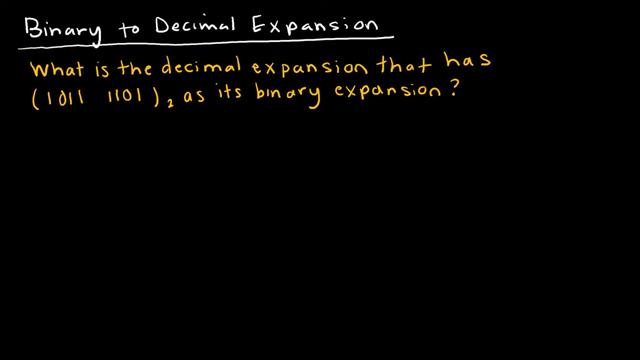 of zeros and ones Again, because base two means I can either have a remainder of zero or remainder of one, And if we're dealing with this, we're going to do the exact same thing we did before. Remember, even though this is not base 10, this is still now base two. So this is two to the zero. 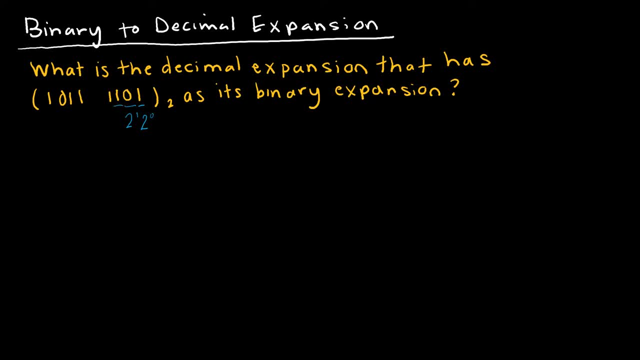 power, And this is two to the first And this is two to the second. And typically what I do- because I'm lazy and don't want to have to write the two that many times- is the zero power: first power, second power, third power, fourth, fifth, sixth, seventh power. 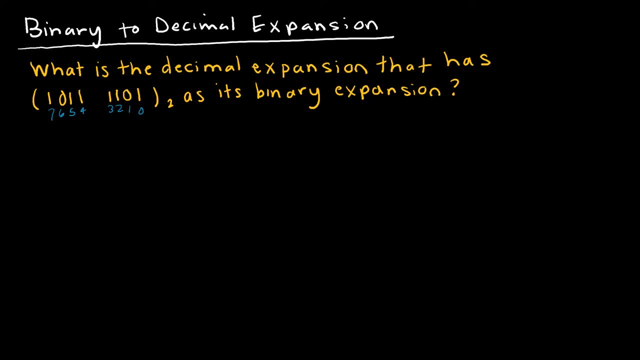 So then, as I am now trying to write this in the proper format, I'm going to say that 10111101, base two- and that's how they indicate base two- can be rewritten as. and then I'm going to look at my first value, which is one. 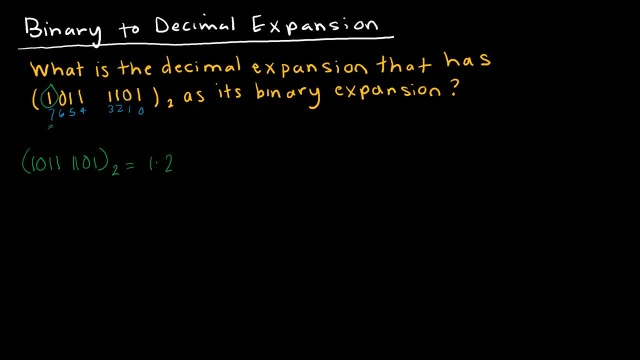 And that's the seventh power. So one times two to the seventh. So those values that I wrote underneath are just the exponents on my base of two, Again two, because it's binary. So then I move on to the next value, which is zero. Zero times two to the sixth, plus one times two to 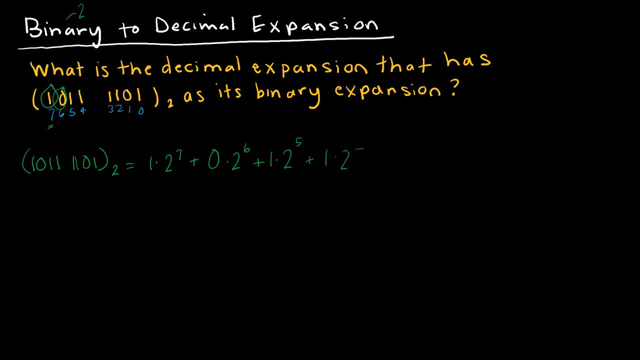 the fifth, plus one times two to the fourth. And again, I'm just looking at these values and these exponents. So I'm going to say that zero plus one times two to the third, plus one times two to the second, plus zero times two to the first, plus one times two to the zero. 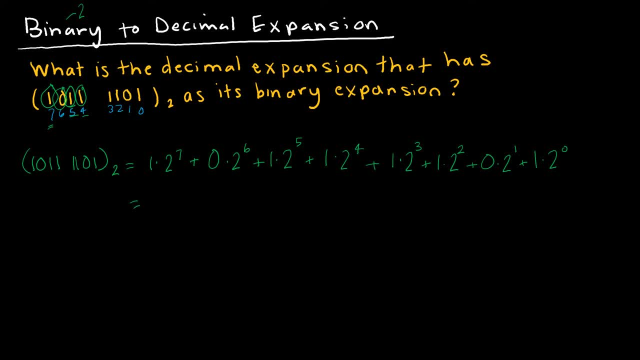 From here I'm going to just do some simplifications. So this is one times 128.. I'm not even going to work with the zero, because who cares? So this is one times 32, plus one times 16, plus one times eight plus one times four. Again the zero. I'm not going. 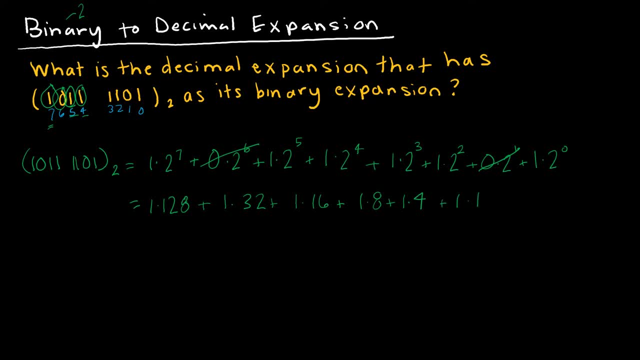 to mess with plus one times one. And if I add up 128,, 32,, 16,, eight, four and one, I get 189.. Now keep in mind it said: write the decimal expansion. And, as I said, 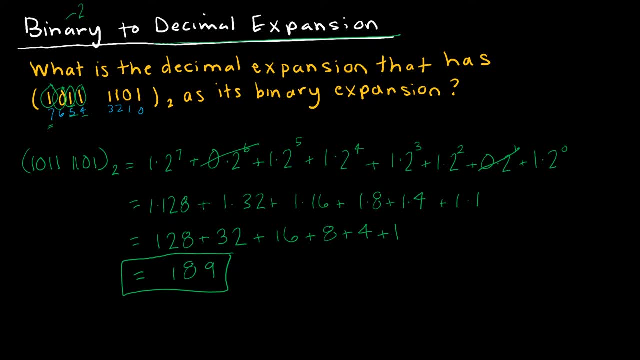 before. if you're writing a decimal expansion, we're not going to then turn that back into 1 times 10 squared, plus 8 times 10, plus 9, because base 10 is the number system that we use. So we're just going to keep it as 189.. 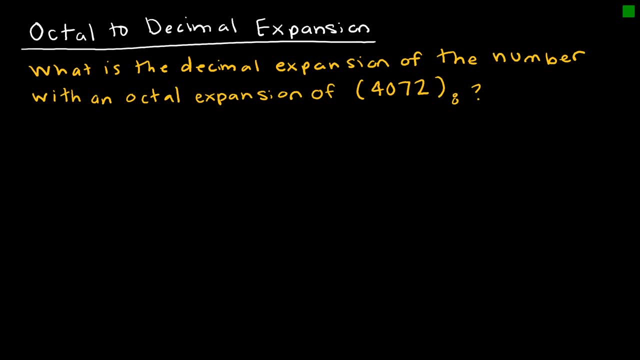 So, the same way that we just did for a binary to decimal expansion, now we're going to look at an octal to decimal expansion. expansion, And, of course, octal means the base is 8.. So here we have the number 4072,, base 8.. I want 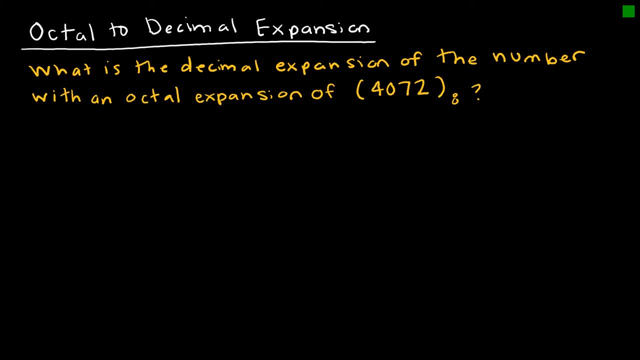 to turn that into a base 10 number. So I'm going to go about it in the same way I did before And remember I start on the right and it's just a good little numbering system to help you know exactly what we're dealing with here. And the numbers that I've written beneath again are: 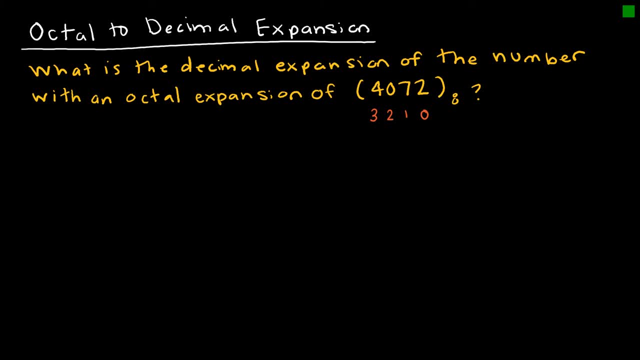 going to be the exponents on the base of 8.. So if I'm writing 4072, base 8, into a decimal expansion, I'm going to say I have 4 times 8 to the 3rd, because 4 is my first digit and 3 was. 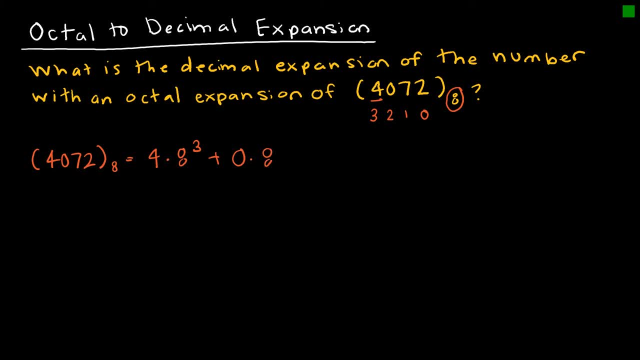 that exponent plus 0 times 8, squared plus 7 times 8.. So I have 8 to the 1st plus 2, and again you could put times 8 to the 0, but we don't have to. 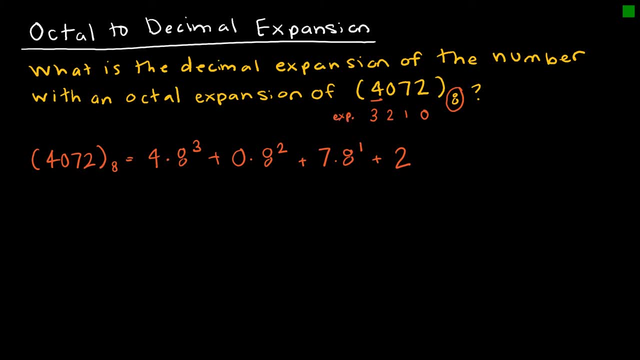 So again, these are just my exponents, and then up here these are the numbers that I'm multiplying. So, just as I did before, you can show that step in between if you want to show that this is 4 times 512. 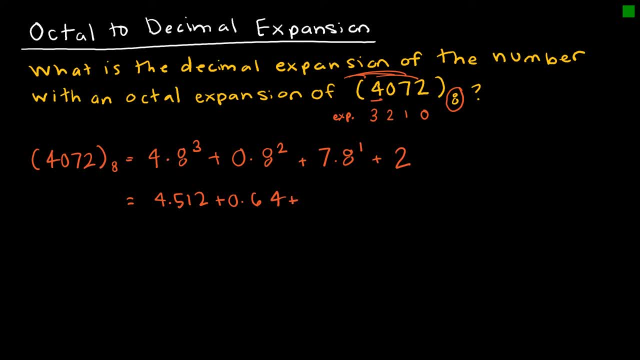 And 0 times 64, and 7 times 8, plus 2,, or you could just go straight to this step, which is to find 2048, plus 0, plus 56, plus 2,, and then my final answer, of course, would be 2106,, and again, this is. 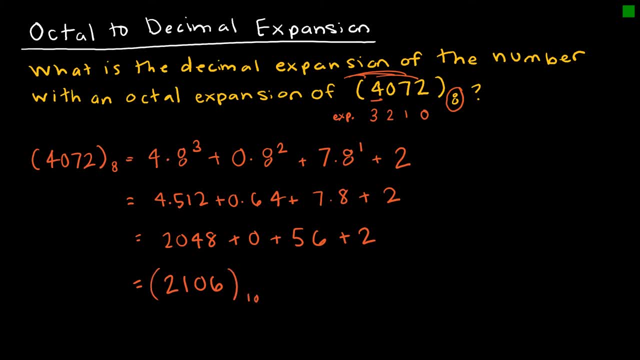 base 10, so it's okay to go ahead and put that base 10.. Keep in mind, when we're dealing with base 10, that it's not necessary. so it's just as acceptable to just write 2106, as we normally would. 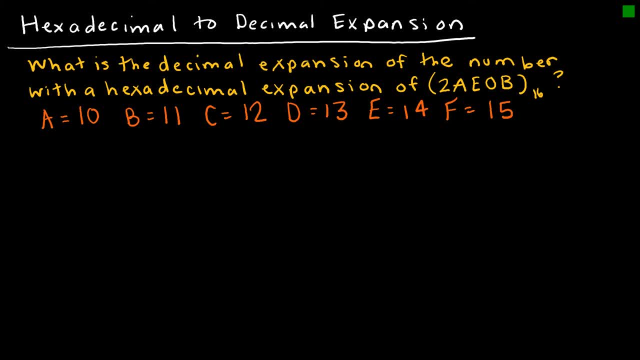 Now let's look at a hexadecimal expansion. Now, hexadecimal again is something we haven't dealt with before, and this one gets a little bit tricky because we're dealing with a base of 16, so hexadecimal means that we're dealing with a base of 16, and the problem with this is obviously when we're looking at one-digit numbers. we've got 0,, 1,, 2,, 3,, 4,, 5,, 6,, 7,, 8,, 9, but when we get to 10, we don't have a one-digit number, because if I wrote 10, that would be two digits. 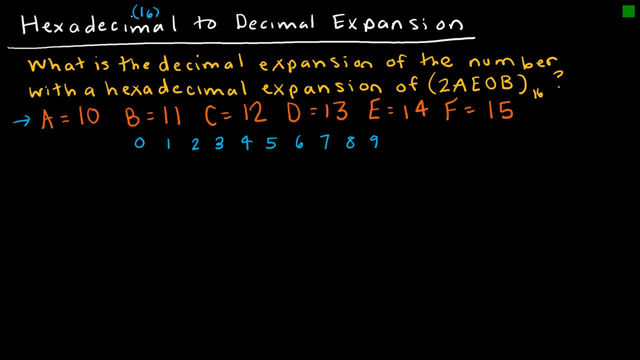 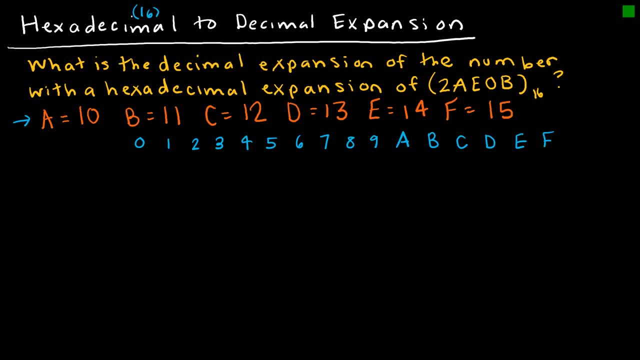 So these are the values that we're going to use for hexadecimal to decimal expansion, But the good news is it's really just exactly the same thing. So, to find my solution, I'm going to just recopy this over here and again. this is base 16, and, just as I did before, I didn't. 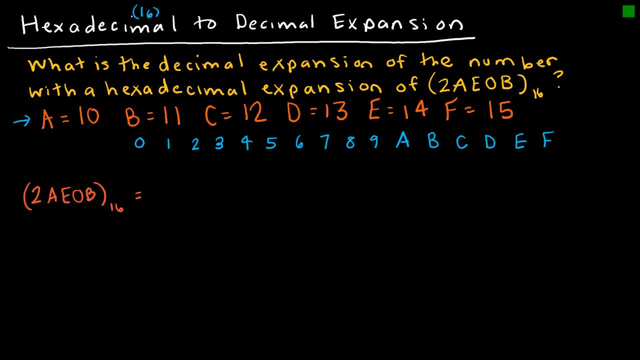 leave myself a lot of room, and I apologize, but this would be 0,, 1,, 2,, 3, and 4, and so I would start with 2 times 16 to the 4th, Because I'm using my first value and then the exponent. 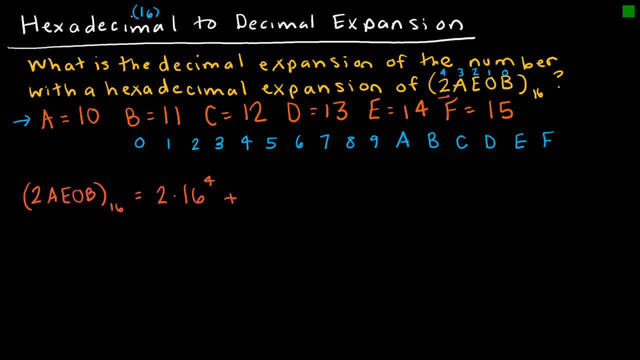 Plus and now I can use A, but A is not A, A represents 10.. So I'm going to say 10 times 16 to the 3rd Plus and now I have E. E again represents the value of 14.. 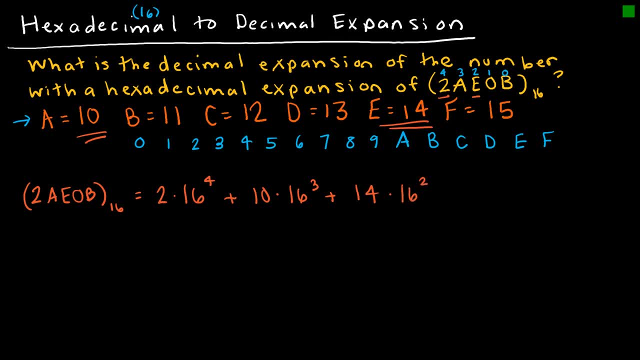 So 14 times 16 to the 2nd, Plus 0 times 16 to the 2nd, Plus B and B is 11.. And so that is my expansion. Again, I can use my calculator to calculate all of these separate values and then at: 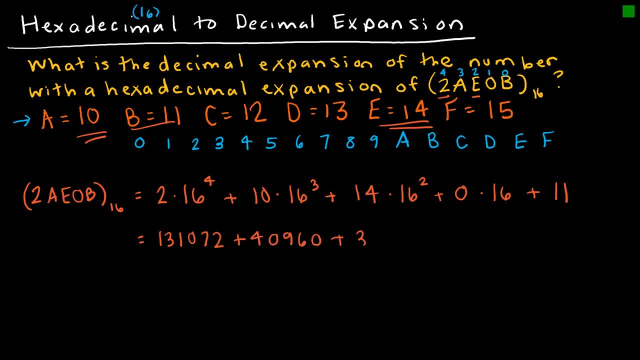 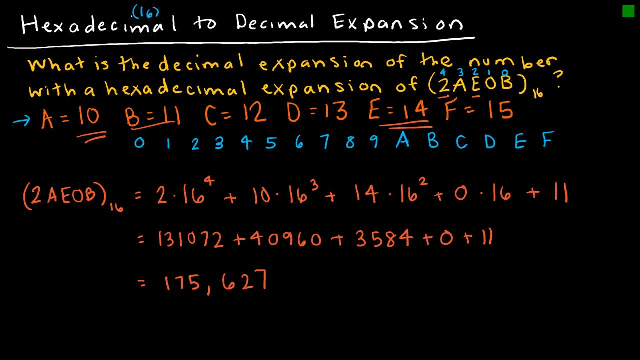 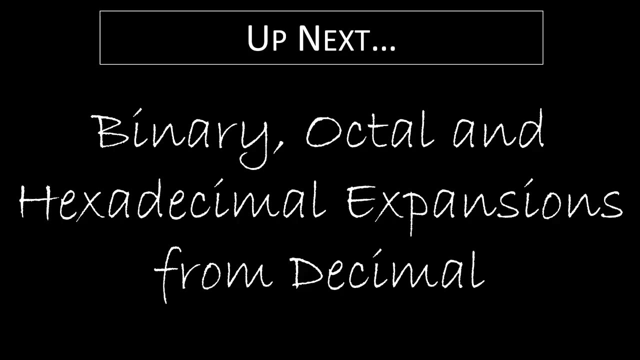 Again, keep in mind I could write that base 10 just to be clear that it's base 10,. Up next we're going to take a look at doing what we just did in the reverse order. So we'll start with a decimal expansion and convert to binary, octal or hexadecimal. Thank you. 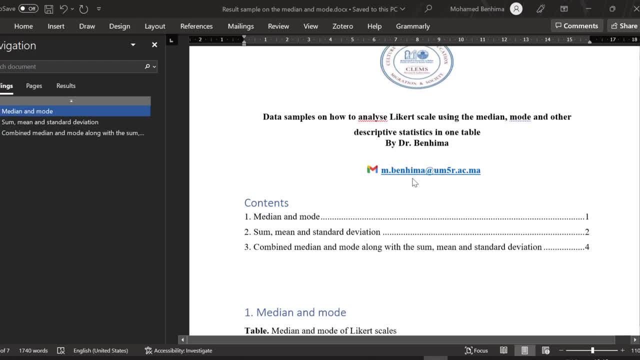 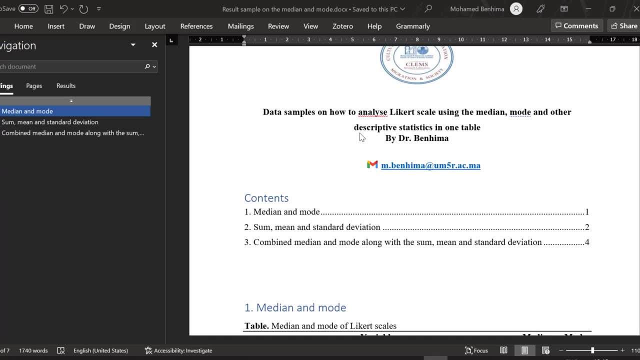 Hello everyone, I hope you are doing great. In this tutorial I'm going to show you how you can analyze Lackert scales using the different descriptive stats, like the mean median mode and other descriptive statistics, in one table. So, as you can see, in this table we have the median 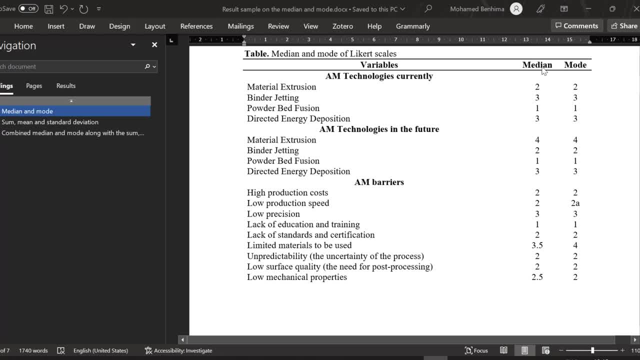 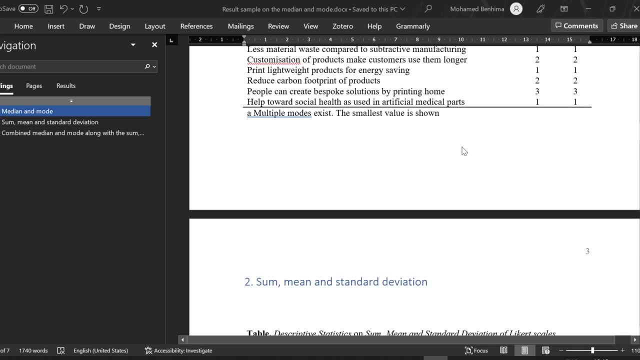 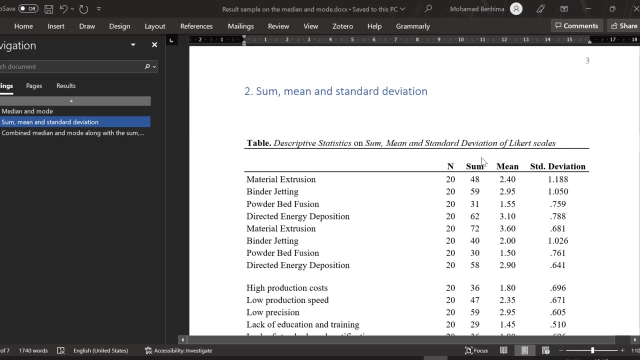 and mode of all the different Lackert scale items. So the median is the mid value, whereas the mode is the most repeated, frequent or frequent value. And then, for the second table, here we have the other descriptives, like the n that refers to the number of the respondents in the sample.